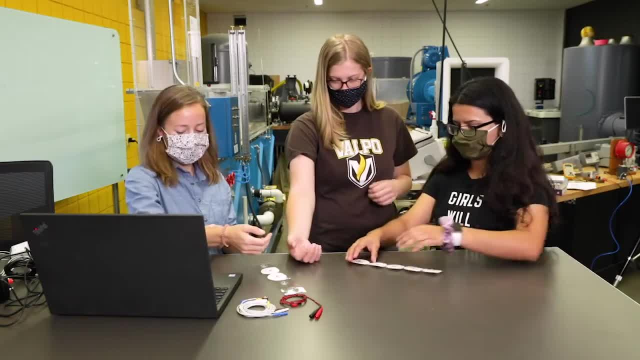 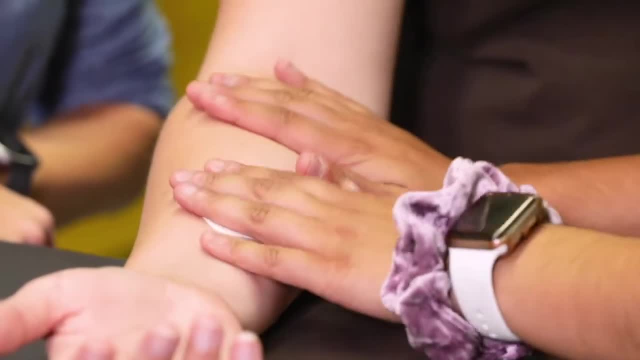 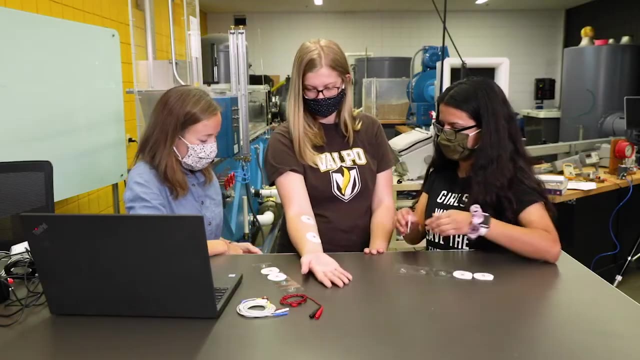 So try and line the electrodes up with the direction of the muscle fibers. It's a little bit far apart, but that's okay, We'll go with it And then we'll put it in. We'll put another one on her elbow for the ground. 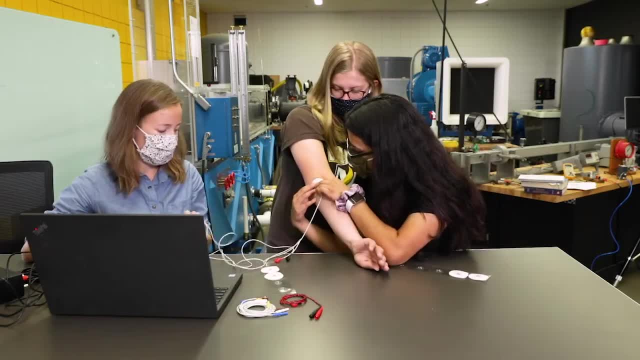 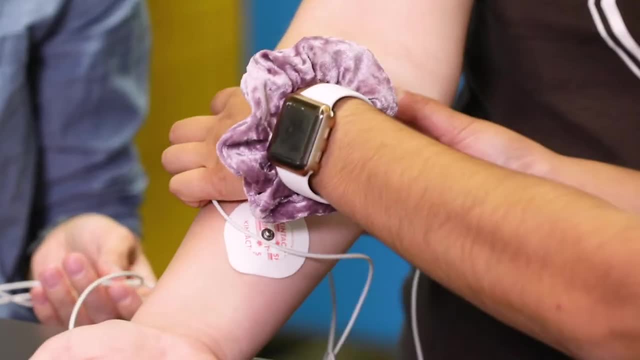 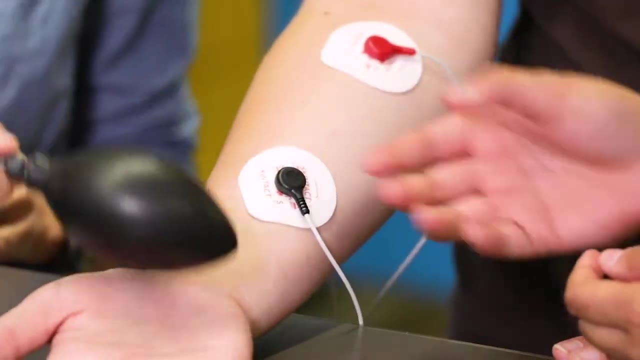 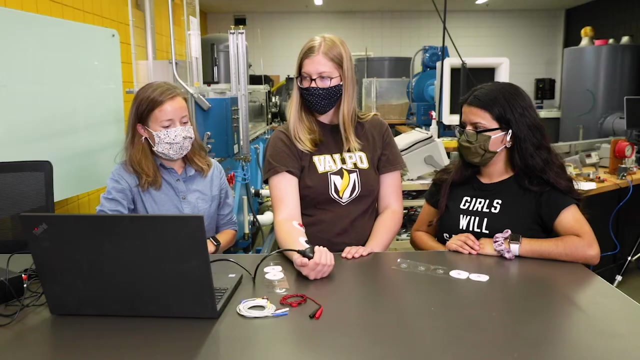 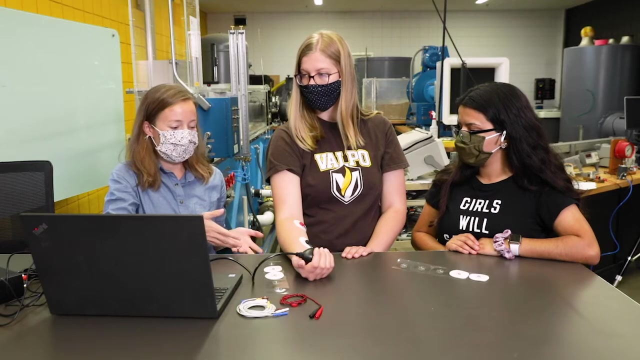 And then we'll connect green to ground And red and black to the other two, All right, and this is going to measure the strength of muscle contraction. So the nervous system is one super cool and complex electrical circuit, And what we're doing here is we're learning about the nervous system and the muscles by recording tiny electrical signals that are given off when muscles contract. 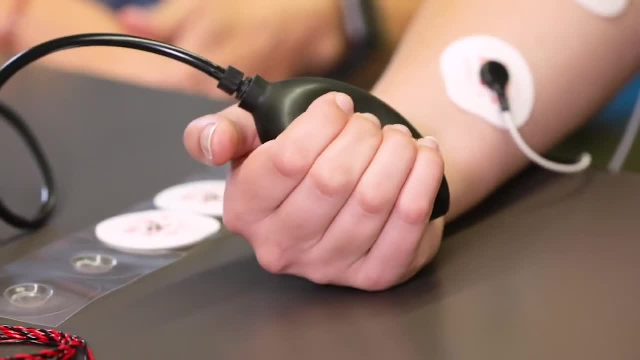 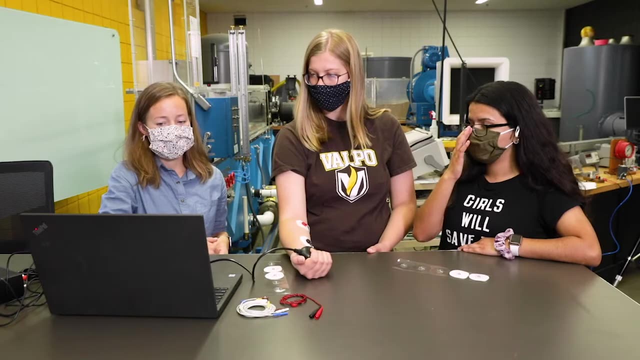 These tiny electrical signals are called electromyographic or EMG signals, So we can use these signals for a lot of different purposes. We can learn about how the brain controls muscles. We can send these signals to prosthetic hands, And we can also use these signals to control someone else's muscles. 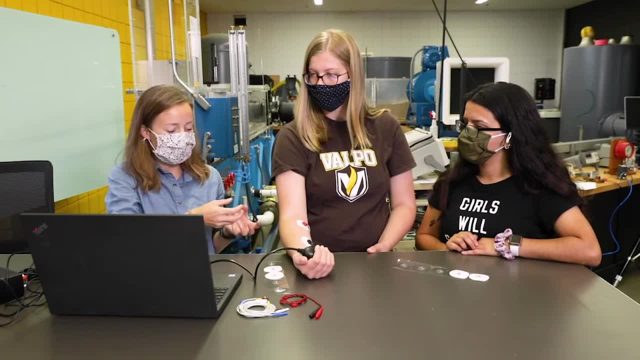 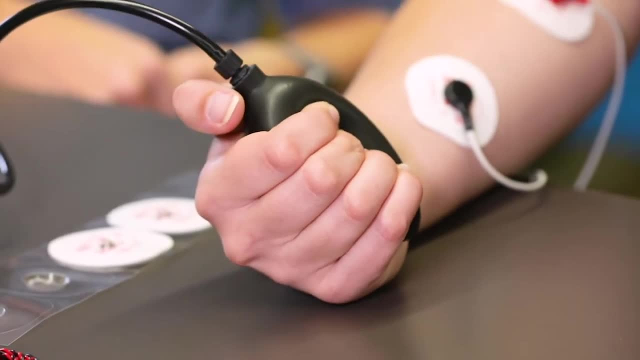 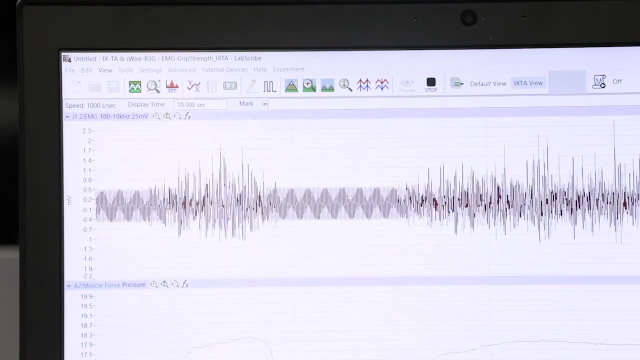 So the same electrical signals that we record from muscles, we can use them to stimulate muscle. So muscle gives off electrical signals and it responds to electrical signals, And we'll show you that in a minute. Oh, that actually looks beautiful, All right. so here on the screen we see the force. 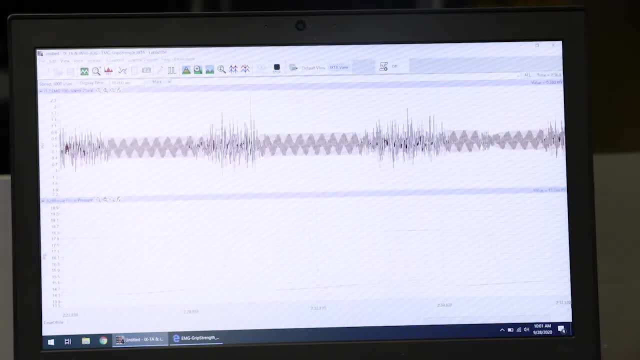 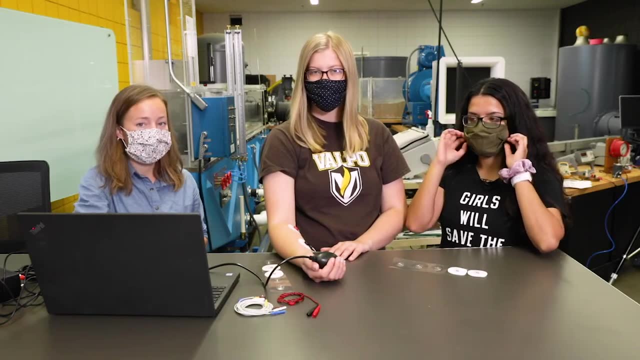 And here we see the force, And here we see the force, And here we see the force. So many of our students are involved in research outside of class And because we don't have graduate students, all of our undergraduate students are the ones that get to present our work at conferences, get to write papers with us. 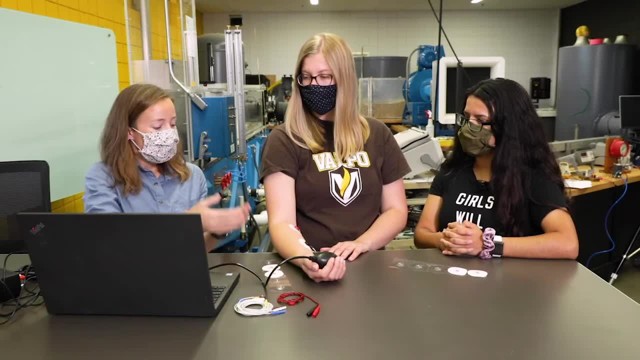 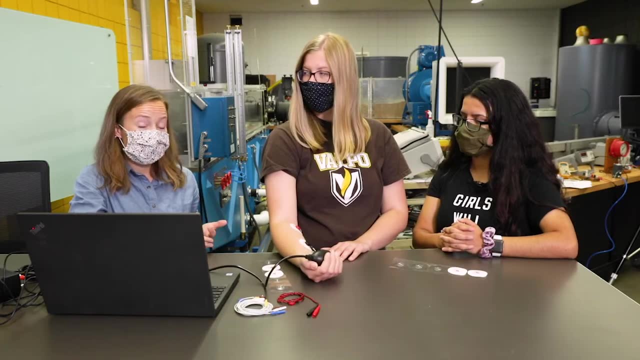 And both Vidi and Abigail are working with us on some research. These EMG signals give us a picture of how muscles are performing and which muscles are firing during movement. That information is really useful in sports as well, And Vidi works on a project involving a lot of muscles. 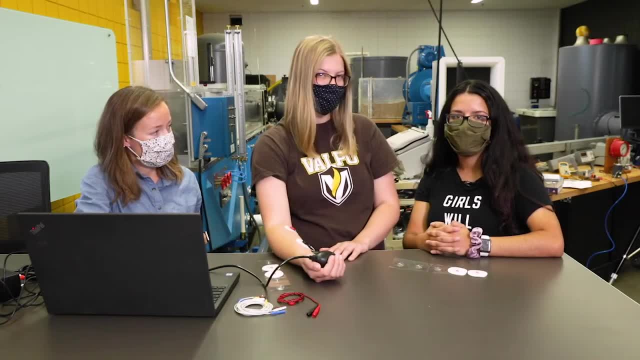 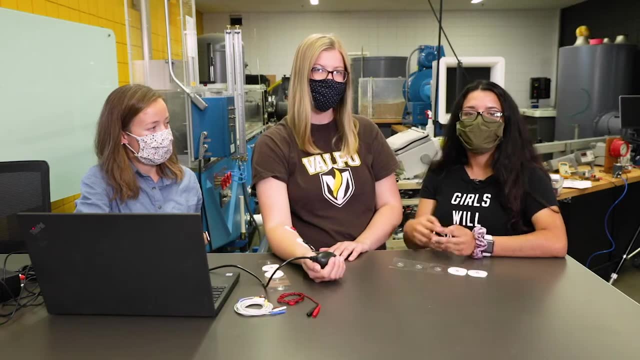 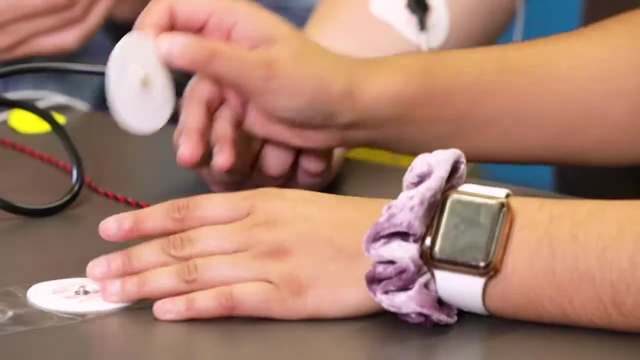 So she's one of our athletes, Yeah, so me and Abigail have both worked on projects involving the NCAA athletes, where we work on injury prevention protocol to help them so they can become better athletes and better perform. So now we're going to use EMG signals from Abigail's arm to control Vidi's arm. 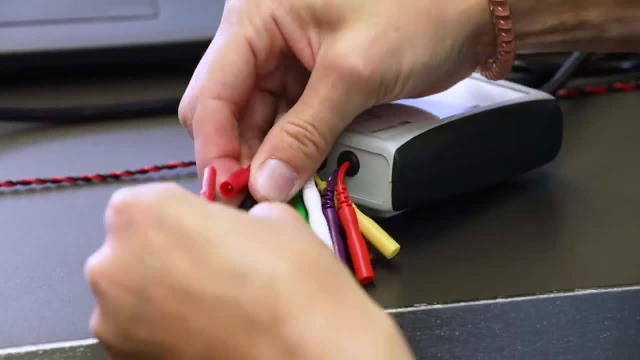 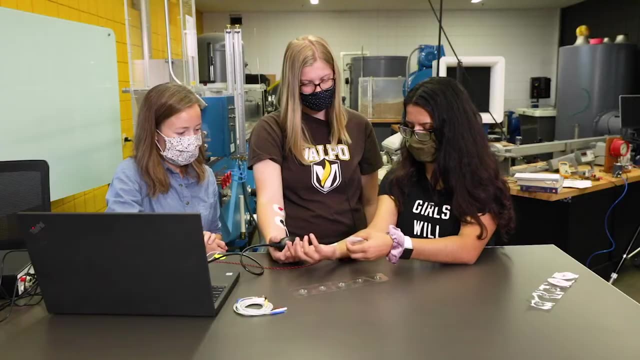 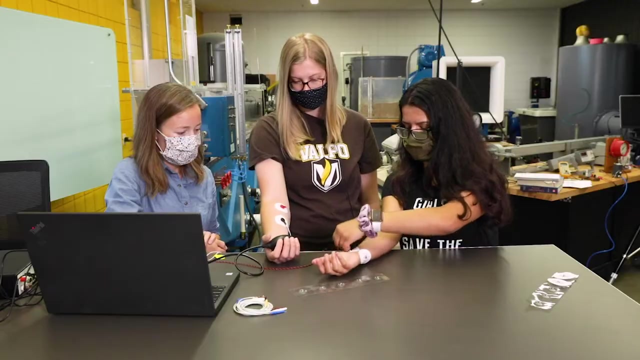 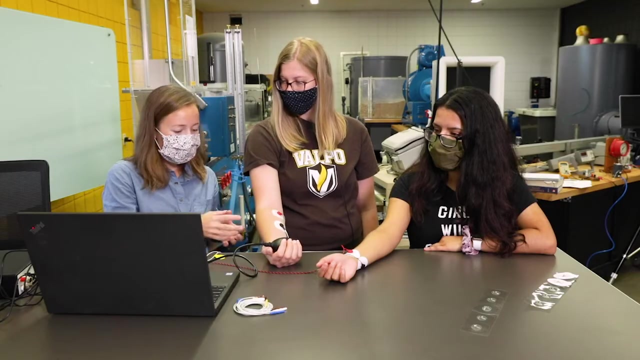 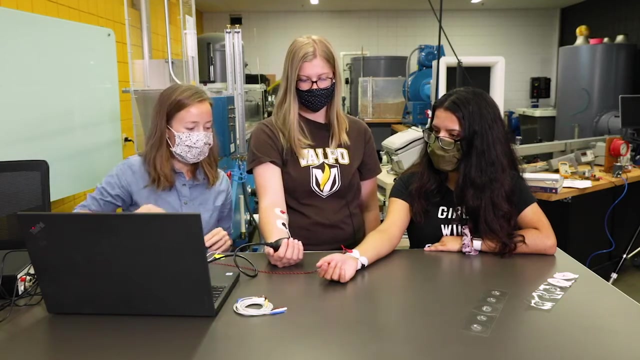 So muscle fibers respond to electricity and they give off electricity. So we can use those EMG signals to evoke a contraction. All right, ready. So these EMG signals from Abigail's arm are sent through the computer, They're processed and then they're outputted as stimulation onto Viti's muscles. 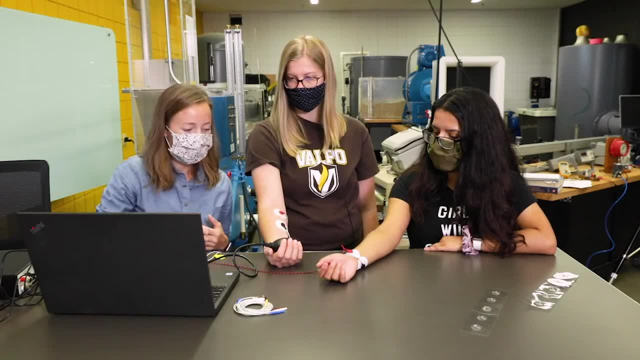 So these signals from Abigail's arm are evoking a contraction in Viti's arm. So when Abigail's muscles fire, the computer is then processing those signals and sending them to tell Viti's muscles to fire. Want to try it? 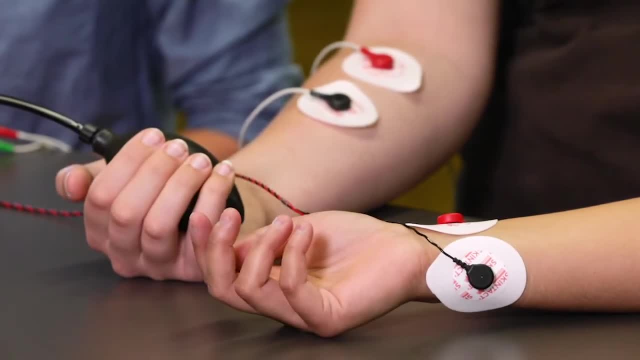 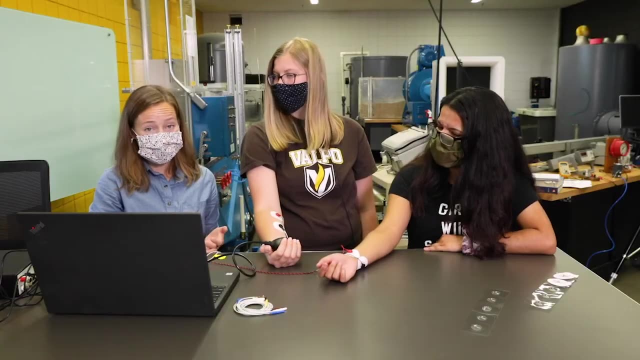 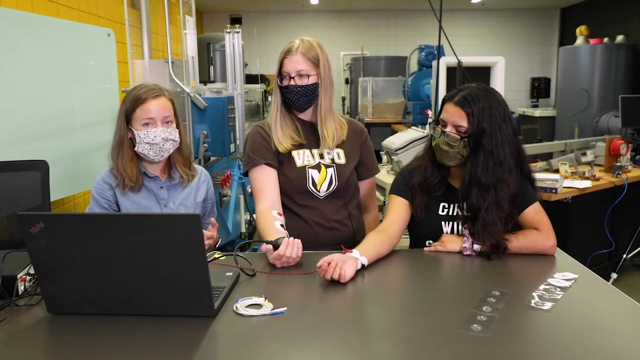 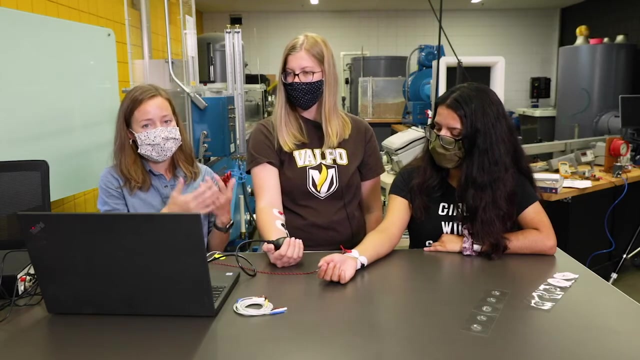 There we go. So because we know that muscles respond to electricity, we can use them for people who are paralyzed or have spinal cord injuries. There's a technique called functional electrical stimulation, which uses signals like the EMG- Viti's EMG signals- to send them to the muscles of a paralyzed person and create muscle patterns. 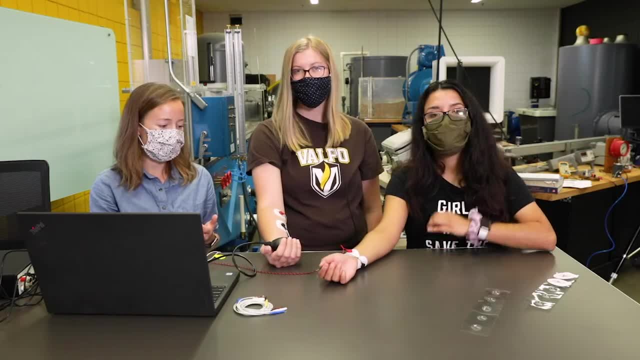 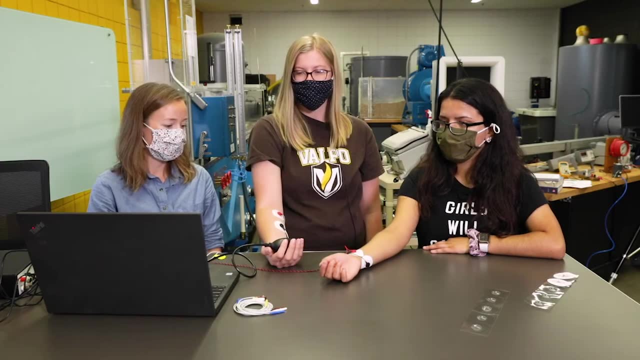 that can be useful for them in completing tasks of daily life. So I actually want to go to school for prosthetics and orthotics. So for me this research is really interesting that I've already got experience with EMG sensors and coordinating muscle movement in people who are paralyzed or in prosthetics. 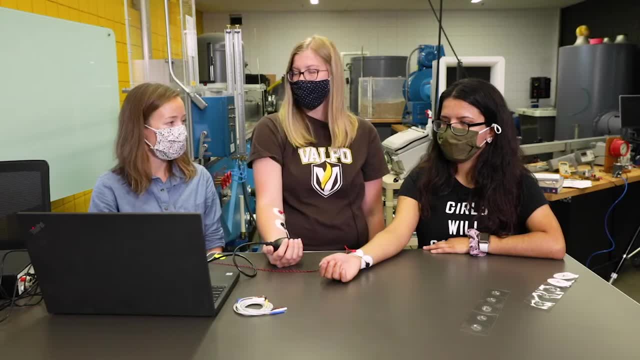 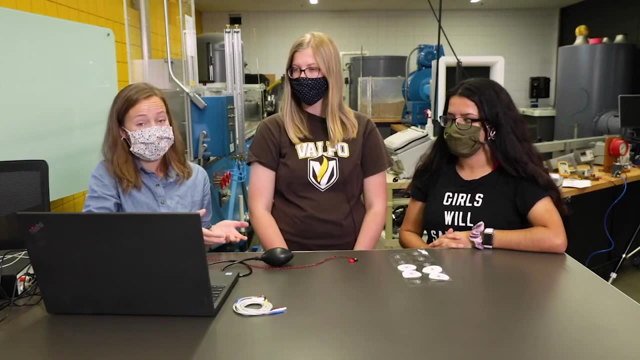 before I even get to grad school. So this will help me be able to effect change for my patients later on in life, before I even get any of that training. So these signals from the nervous system are just some of the signals that we can record. 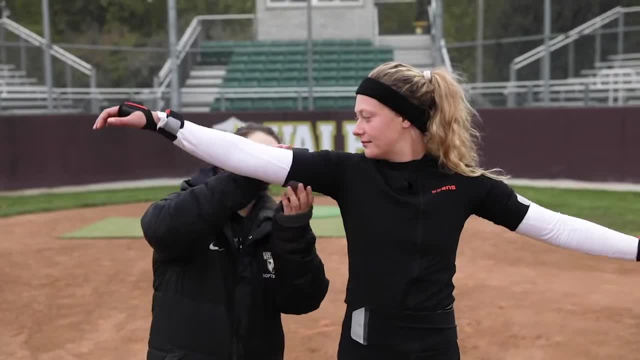 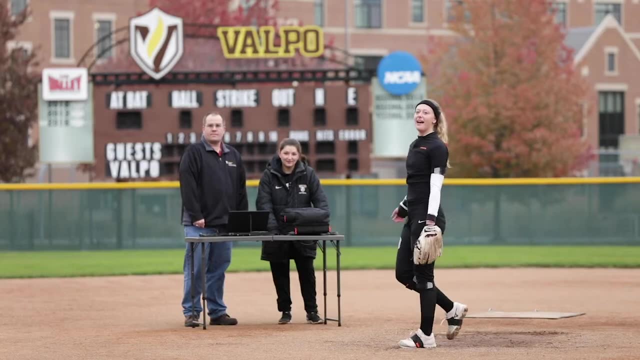 from the human body. We can also record joint angles, velocities and accelerations and we can use that again in something like athletics: to measure human movement, to try to prevent injury, to help people recover from injury and to improve athletic performance as well. 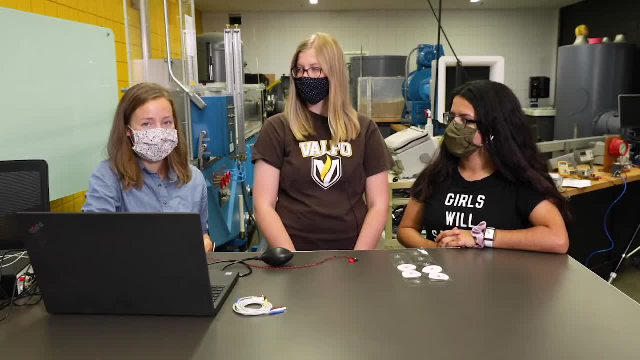 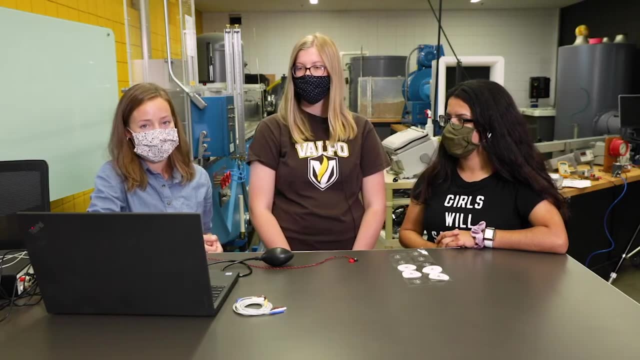 So bioengineering is such a broad field that we've created three tracks. We've got a biomedical track, biomechanics and bioelectrical track, So students can specialize in the type of bioengineering they're most interested in. Students in the biomedical track are really well prepared to go to medical school or graduate. 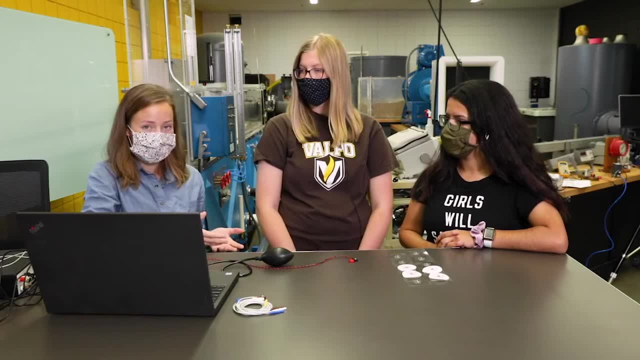 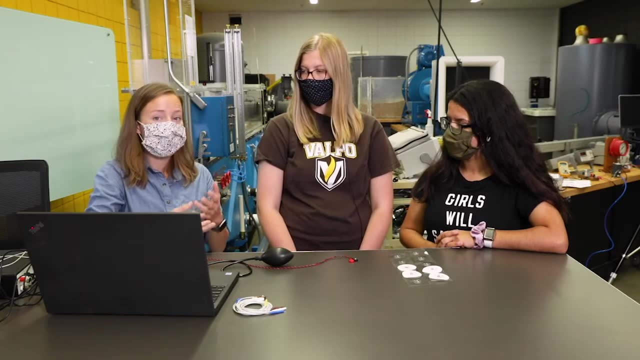 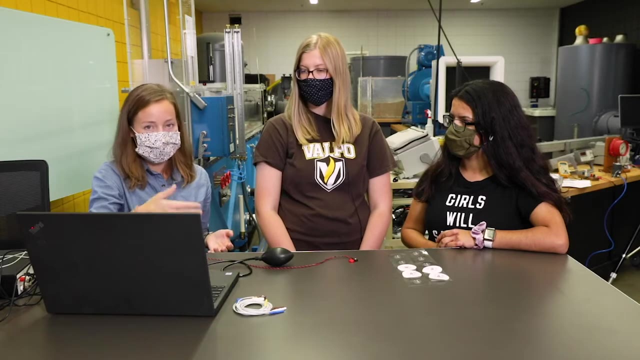 school Students in biomechanics get most of the same classes as a mechanical engineer, and then they get biology and chemistry classes to help them with the application of mechanical engineering to the human body. And the bioelectrical students are similar. They take many electrical engineering classes along with their physiology and chemistry. 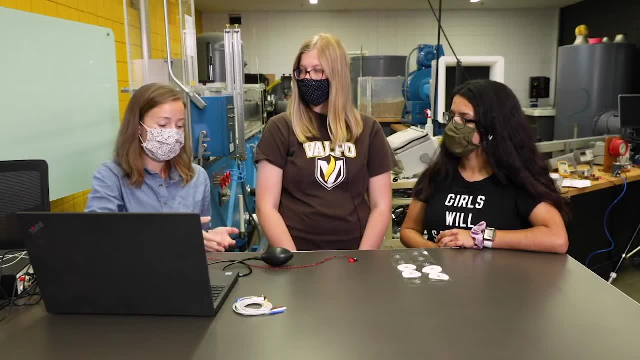 classes to help them look at things like the human nervous system and these electrical signals that we're recording from the human body. So these are some of the things that we're interested in. So part of the engineering curriculum is that we have a senior design course, so you get. 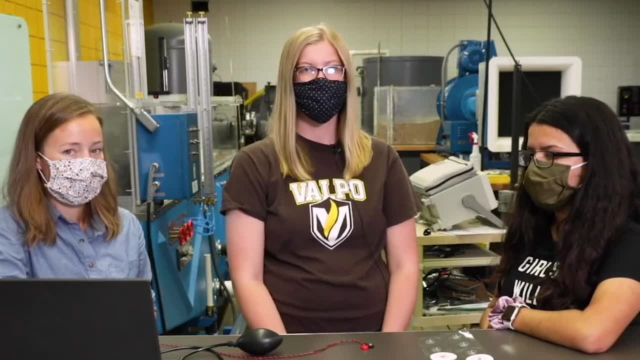 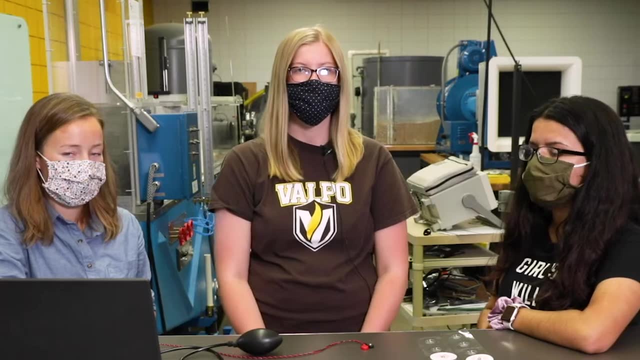 a whole year to design a project. So one of them is to work with physical therapists and outside resources to redesign the mechanism of reciprocating gait orthosis, And so I really get to apply all of the engineering skills that I've learned so far throughout. 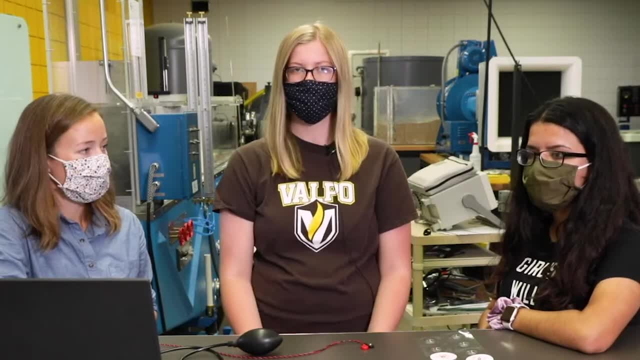 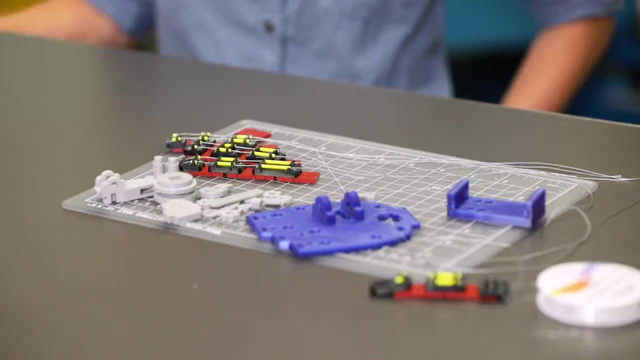 my courses here and get to do a real-world application that's going to be able to help so many people in the future. We can also use EMG signals to control prosthetic hands, So here we have a prosthetic hand that we're building. 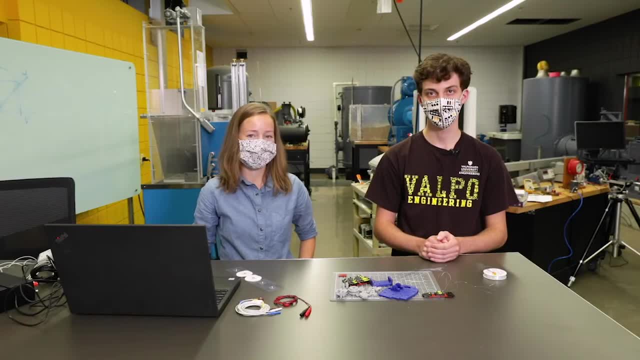 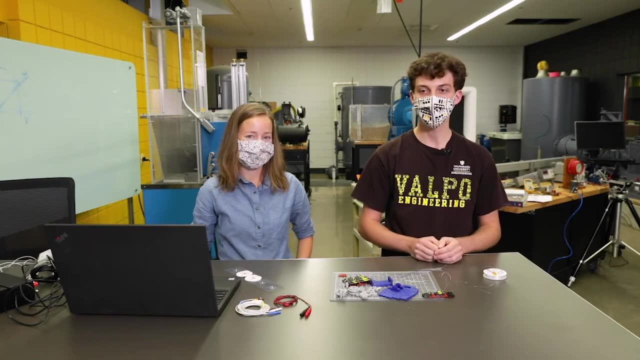 And Carter is one of our bioengineering students who's working on this hand. My name is Carter McCullough. I am a senior bioelectrical engineer here at Valparaiso University and I am a researcher here at the Human-Machine Interface Lab. 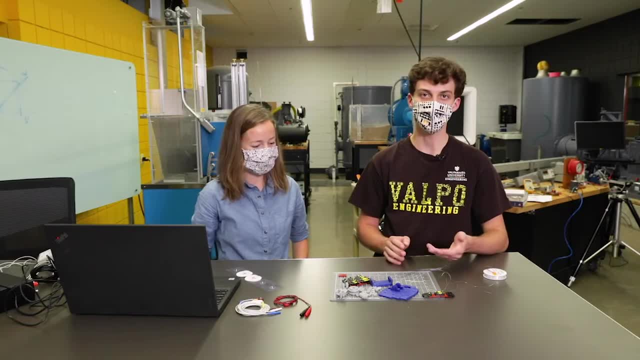 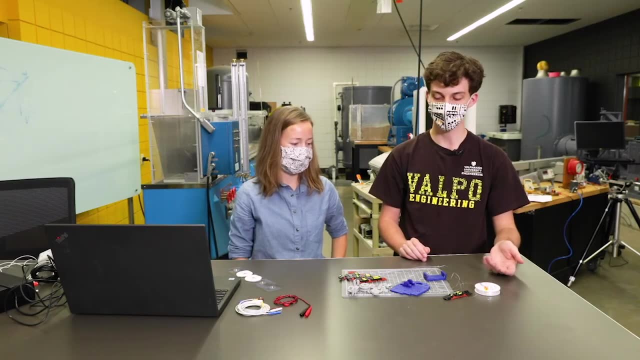 Here I have a prosthetic hand that I built and I will now demonstrate a little bit how it works. So I gathered all these parts from the GitHub page that we received the parts from, And what it is is. you're going to get some fishing line and some other household equipment. 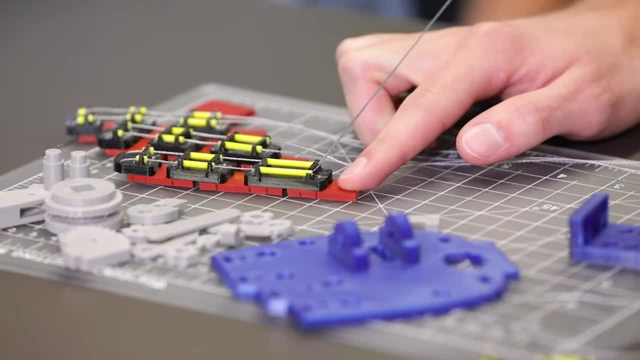 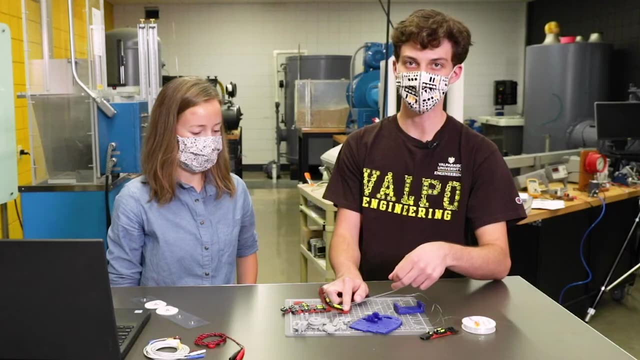 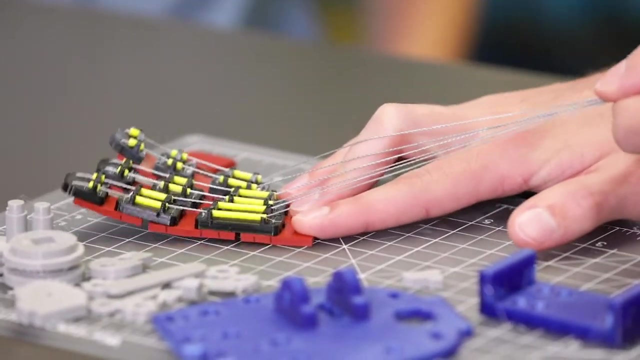 household items with the 3D printing and we're able to create these tendon-like structures within the finger. So when you pull these, it actually creates a motion much like your finger would if you were flexing it. So I'll be taking all of these tendons that I have built and if you pull on them, which? 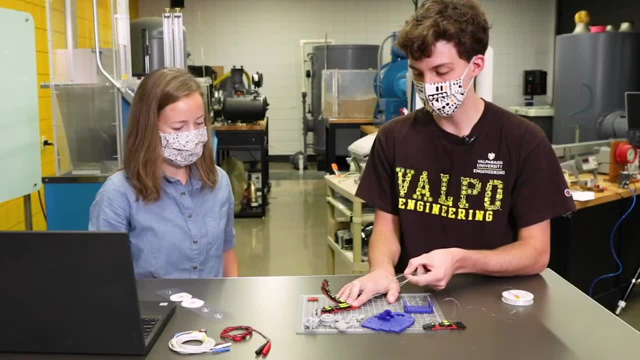 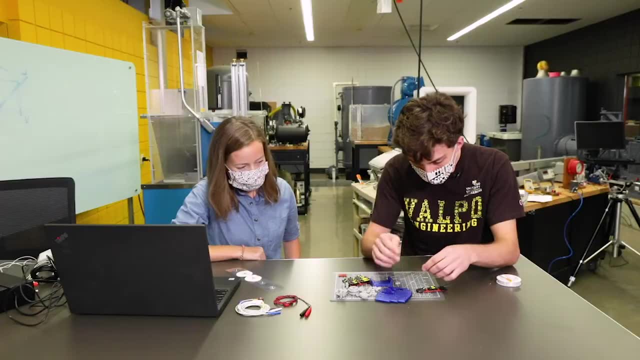 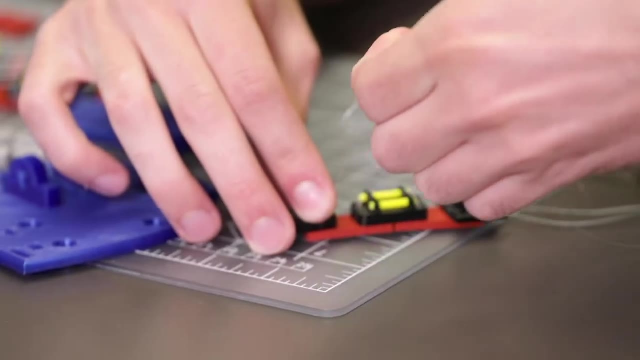 is what a motor will eventually be doing. I'll be able to create a motion with the fingers, much like a human would, And here's how we assemble it. So let's see. So I'm going through here. Looks like actually, for this stitch, all I need, so like, yeah, you just basically weave. 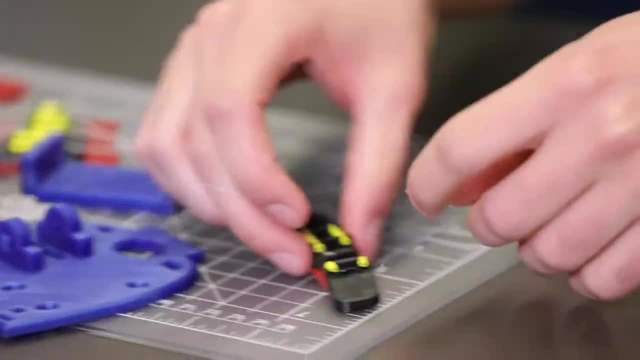 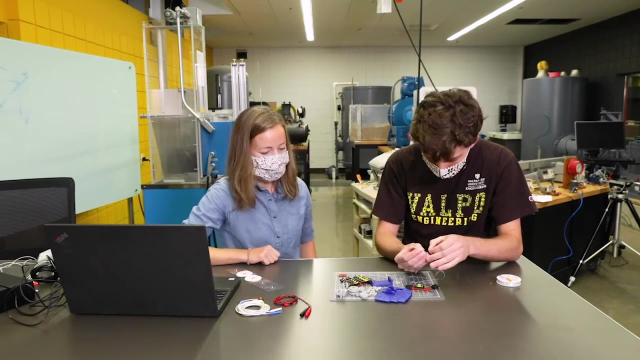 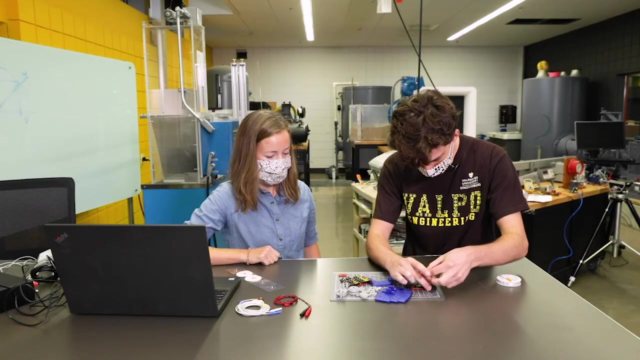 it through here. All right, Okay, So I'm going through. So that's how all of these parts are connected. then, Yeah, that's yeah, they're all connected by stitching And I'll thread this through here And then line that up. 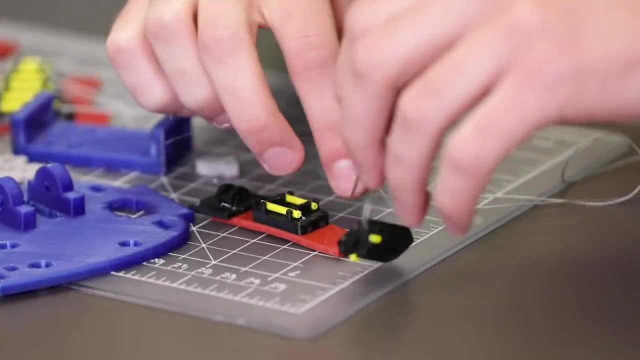 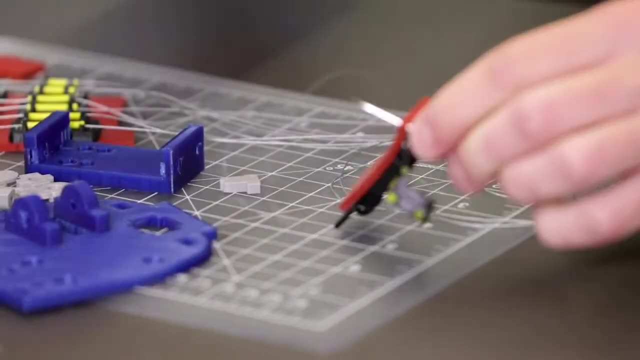 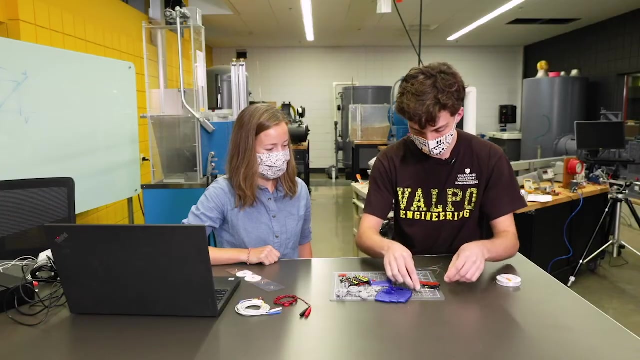 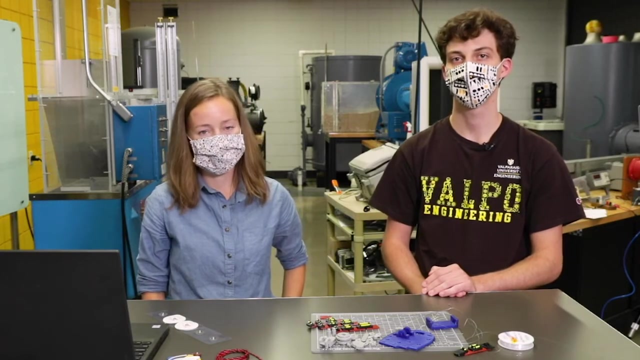 Okay, Hook it through, And this would be a lot easier to do if this needle went through the actual 3D part, but it doesn't, unfortunately. That's okay. So once we have this hand built, students can test out different control methods for. 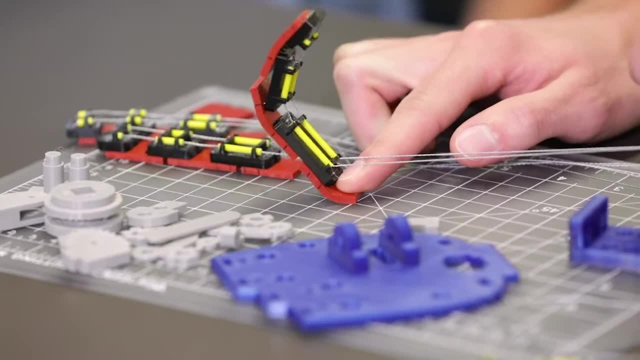 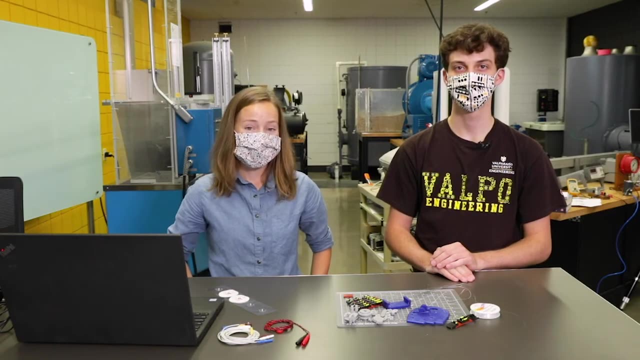 the hand, different ways of mapping EMG signals to hand and finger movement. Okay, These are just a few of the tools that we use in bioengineering, and there are many problems left to solve. So thank you for watching. I'm looking forward to talking with you soon. 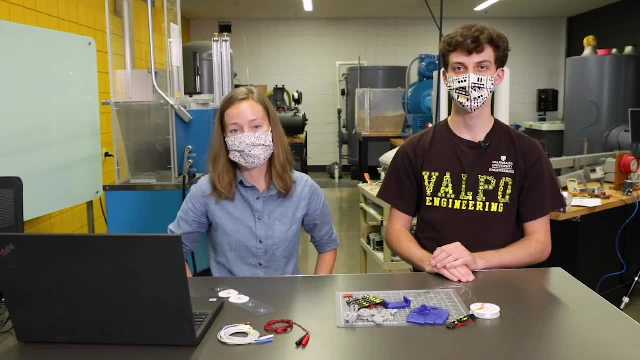 And hopefully we'll get to see you on campus and we can test out some of the signals on your own muscles soon. 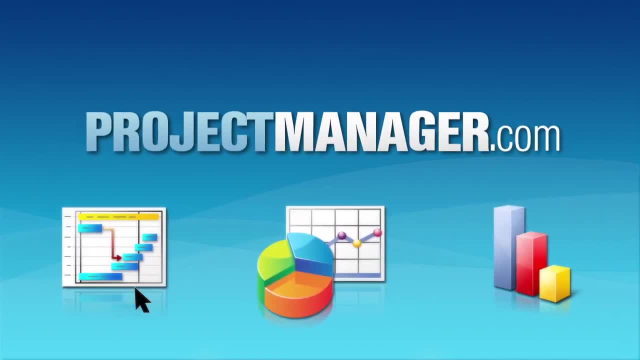 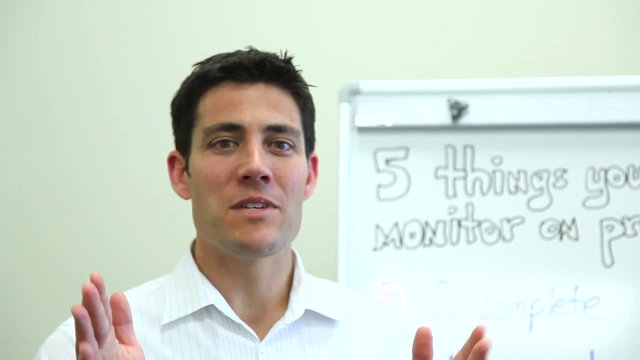 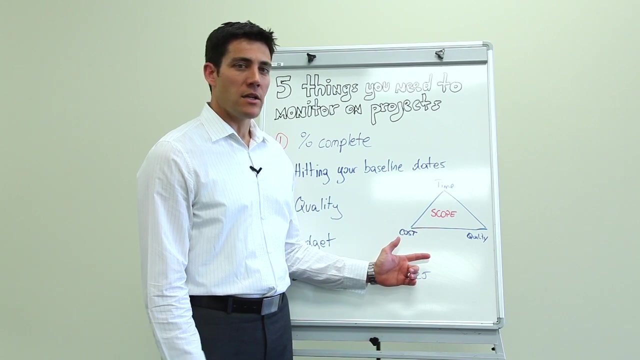 Hi, I'm Devin Dean Content Director here at ProjectManagercom. Today we're going to talk about five things you need to monitor on your projects. Now everybody knows about the triple constraint- of time, cost and quality- governing what you can deliver on scope. but